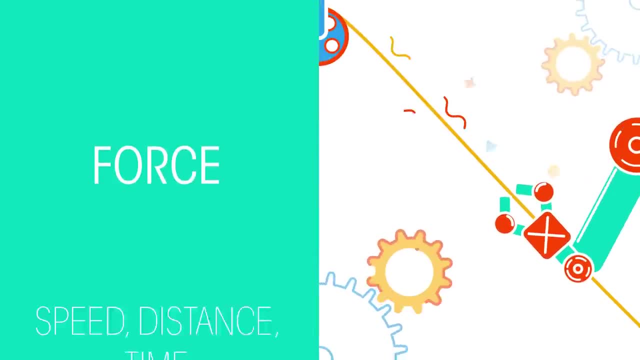 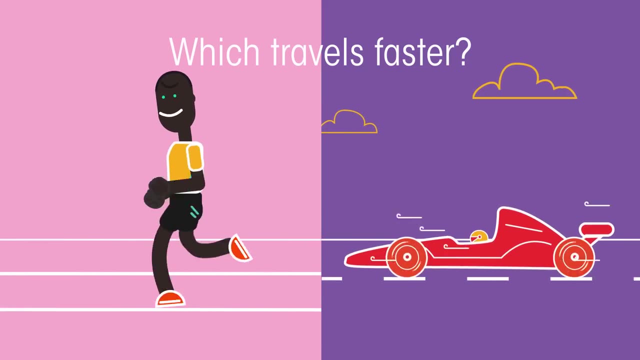 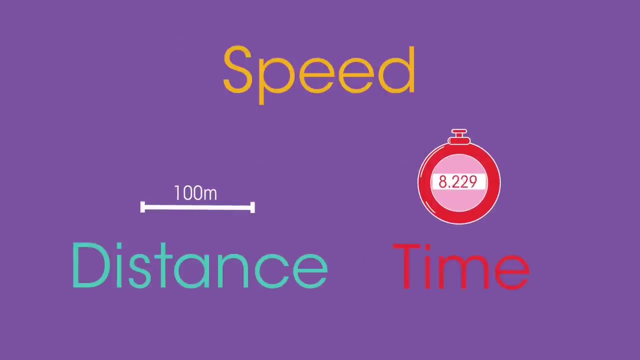 Which travels faster- Usain Bolt or a Formula One car? In this video, we'll find out how to calculate speed using distance and time, which we'll then use to work out the answer to who's faster. Speed is a measure of the distance an object travels in a certain time. Speed can be calculated using 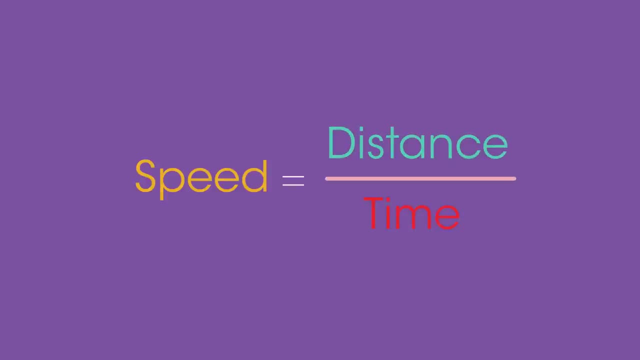 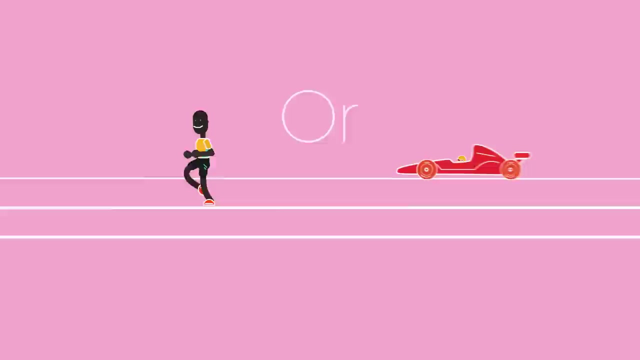 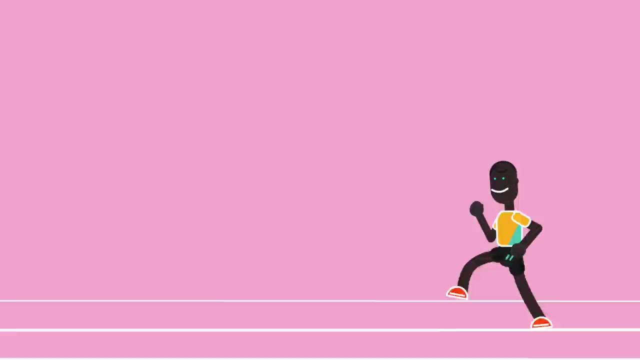 the formula speed equals distance traveled divided by time. So to work out which is faster, Usain Bolt or the F1 car, we need to know how far they both traveled and how long it takes them to cover that distance. Let's work out the speed of Usain Bolt first. In 2009,, Usain Bolt set the 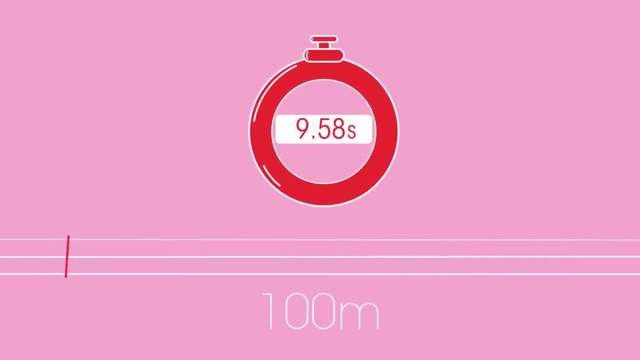 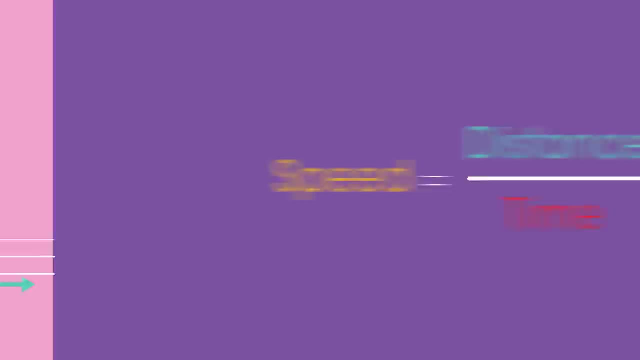 world record for the 100 meter sprint in 9.58 seconds. The distance was 100 meters. The time taken was 9.58 seconds. Using the formula of speed equals distance divided by time. 100 meters divided by 9.58 seconds means his speed was 10.44 meters per second. We have the units for distance. 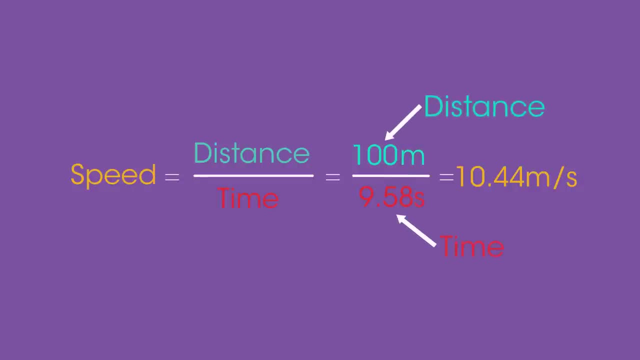 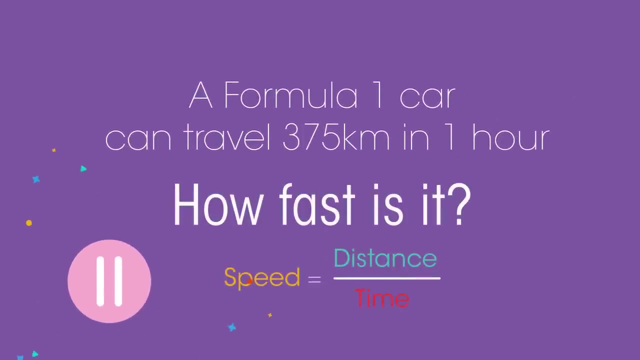 and time meters and seconds which we use to work out the units for the speed Meters divided by seconds, which we say as meters per second. That's pretty impressive, even for the fastest man on earth. So how fast is an F1 car for us to compare him? to Pause the video and work it out. 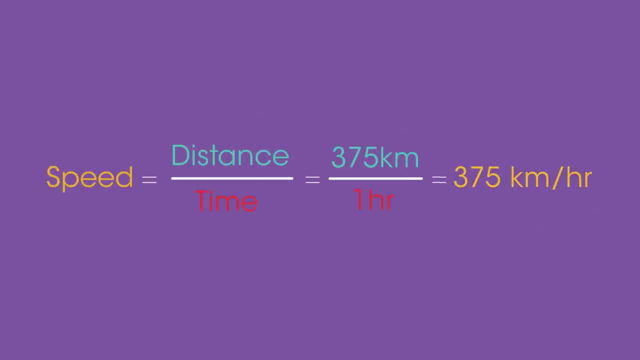 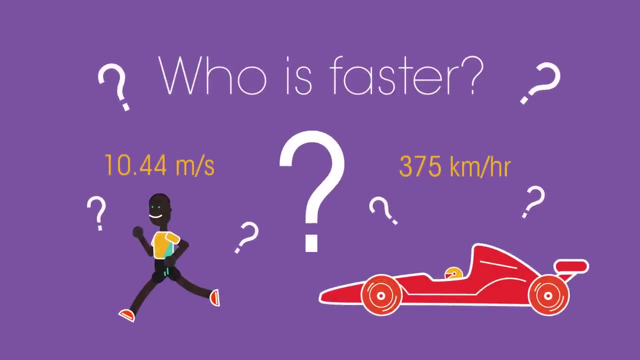 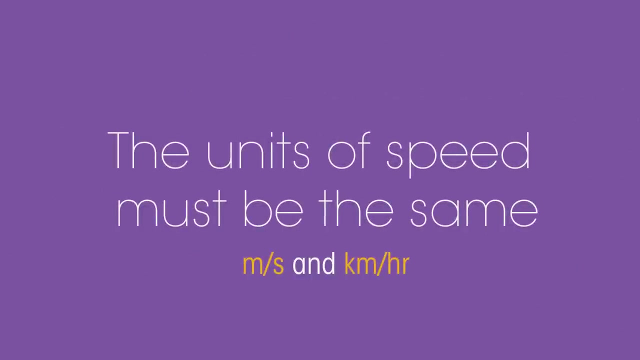 Did you get 375 kilometers per hour? So who's faster? Hmm, from these speeds we can't tell. What's the problem with comparing these two answers? Pause the video and have a think To work out which is traveling faster. the units of speed must be the same, So let's convert the formula. 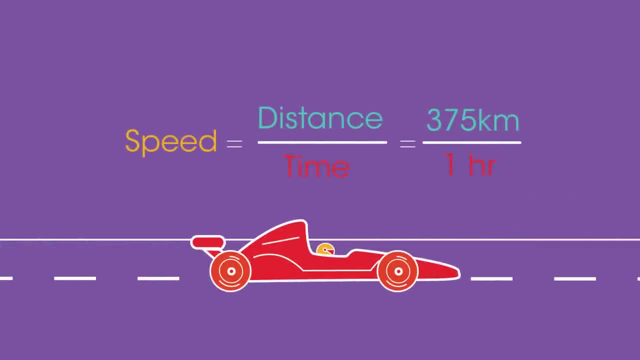 one speed also into the speed of the F1 car. The speed is again 1.20 meters per second. Kilometers into meters multiplied by a thousand, and turn one hour into seconds, by multiplying by 60 for minutes and then 60 again for seconds. So 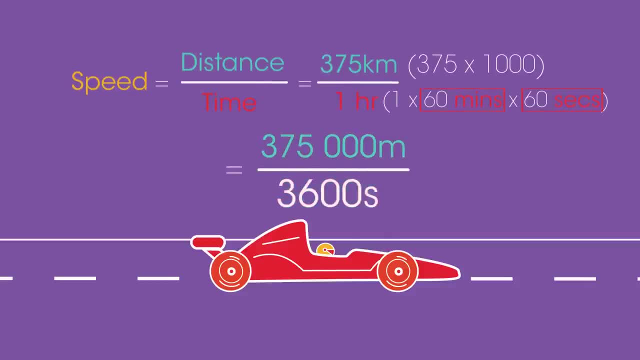 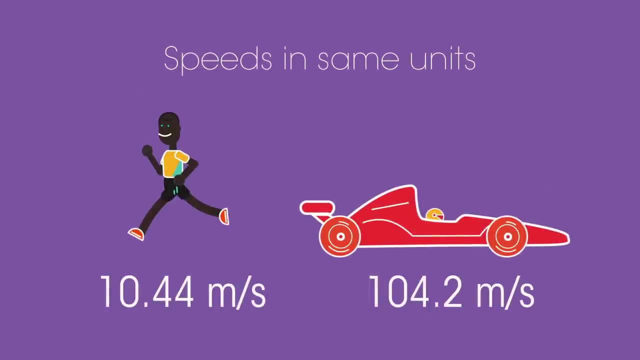 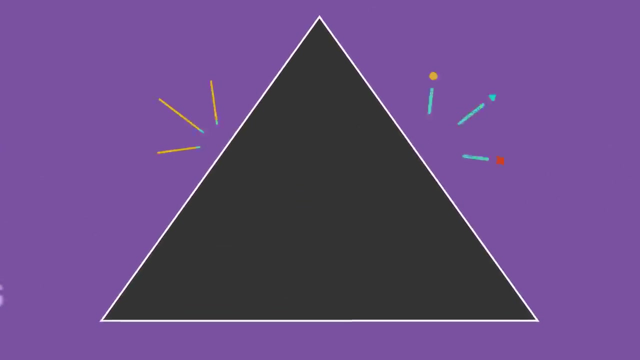 375,000 meters divided by 3,600 seconds gives us 104.2 meters per second. Now we have our speed in the same units. it's easy to see that the Formula one car is much, much faster. The formula can also be written in a formula triangle: